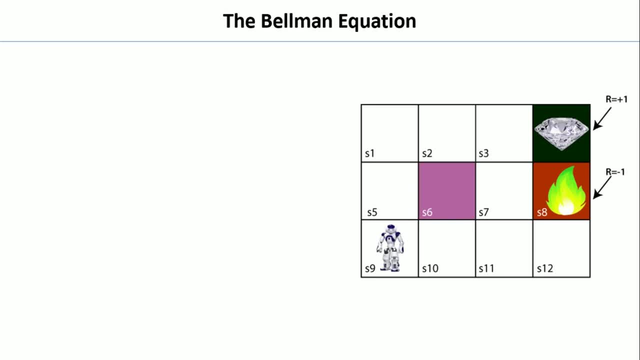 situations. So we need to assign some different values for different cells here, based on where that particular cell is present. For example, if a cell is present close to this particular goal, we have to assign a maximum value in this case. This is the grid I am going to consider. for this example, The grid consists of three rows. 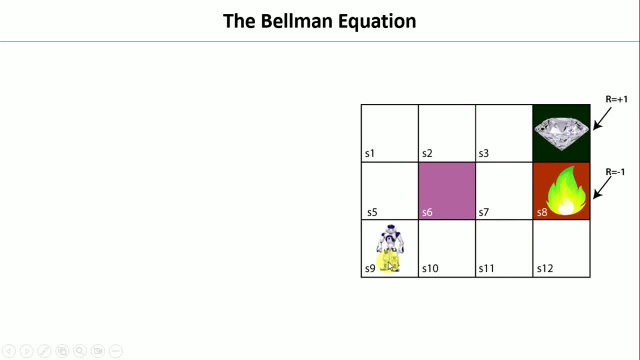 and four columns. The robot is: are the agent is present in s9, s6 is the block here, A seat is a danger or a fire. whenever agent goes here, it will be given a reward of minus one, and s4 is the goal here- and whenever agents come to this one, it will be given a reward of plus one. over here. now what? 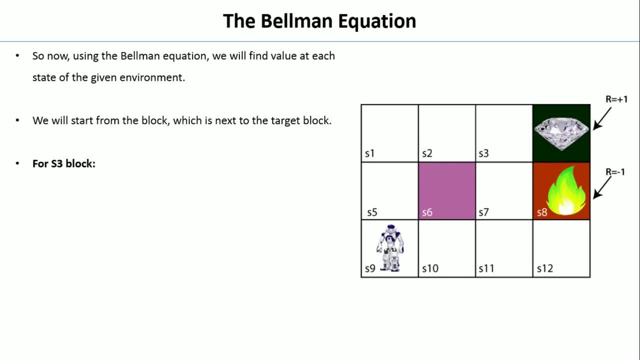 we do is we will start from a cell which is next to this particular goal state here, that is s3. now, whenever you perform an action, that is the right moment, it will go through this particular goal. so that's the reason it will be given a reward of a plus one over here. 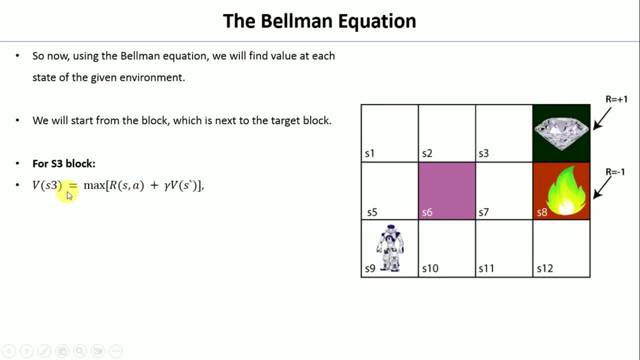 the equation for uh bellman equation looks something like this: v s3 is equal to maximum of rsa plus gamma v s dash. so in this case rsa is equal to 1, because you will get a reward of 1 whenever it goes the right side. here, gamma is equivalent to 0.9. we will consider just for. 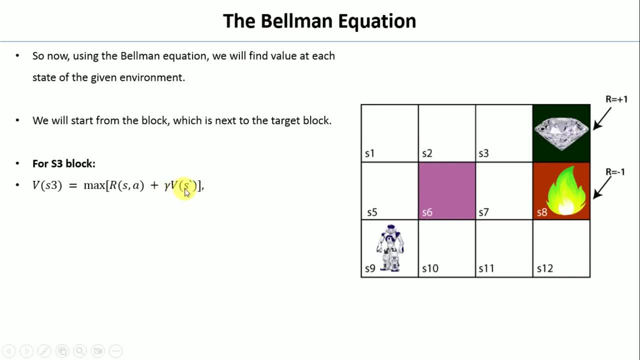 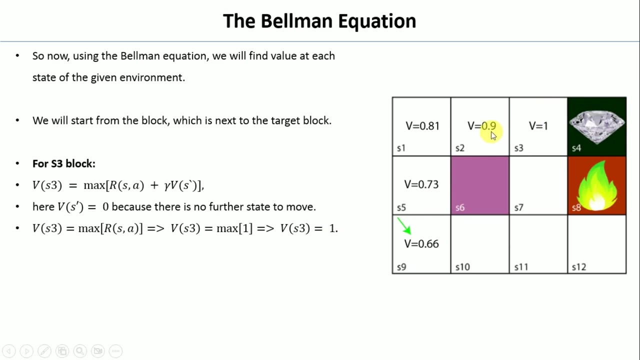 understanding purpose, that's a discount factor and v s dash is equal to 0 in this case, because this is the first state or the transition we have performed here. so if you put all those particular values, phi s3 will become the one in this particular case, so i will put that particular one over here. similarly, i 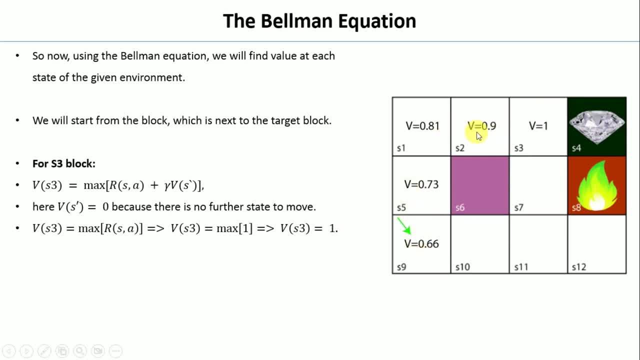 have written the values for other states also, we will try to calculate step by step. in this case, now we have done with s3, we will try to calculate the value for s2. the same equation we will use, that is, phi. s2 is equivalent to maximum of rsa plus gamma or phi s dash. so in this case rsa will. 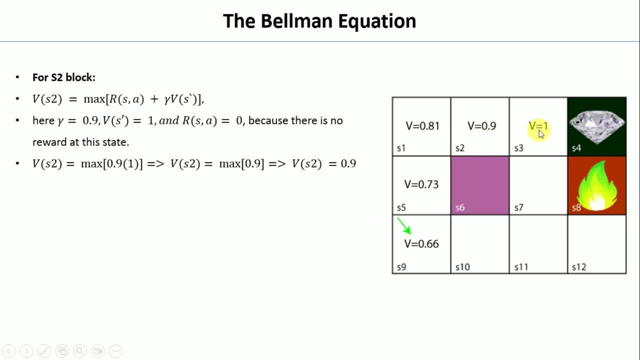 become zero because whenever you perform a right action, you don't get one here, because if you go through this particular goal you will get one, but right now you are going to s3 here. so that's the reason rsa will be zero. as i said earlier, gamma is equivalent to 0.9 phi s dash. that's a previous 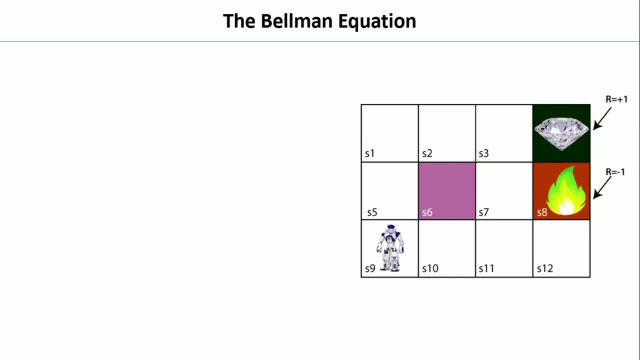 it will be given a reward of minus 1, and S4 is the goal here, and whenever agents come to this one, it will be given a reward of plus 1 over here. Now what we do is we will start from a cell which is next to this particular goal state. here, that is S3. Now, whenever you perform an action that 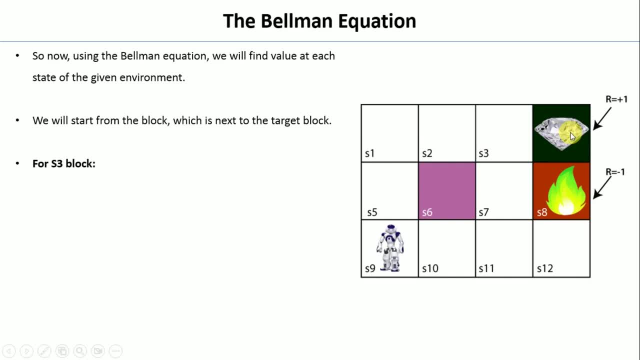 is the right moment, it will go through this particular goal, so that's the reason it will be given a reward of plus 1 over here. The equation for Bellman equation looks something like this: phi S3 is equivalent to maximum of RSA plus gamma Vs dash. So in this case RSA is 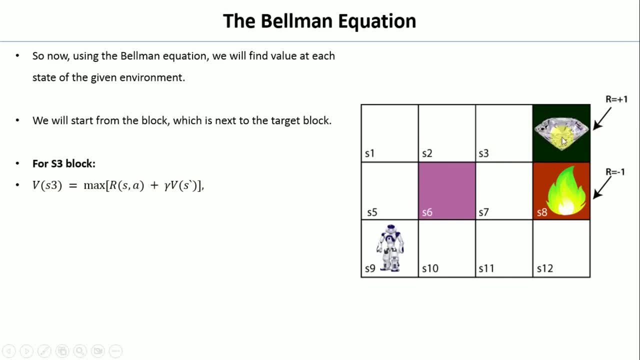 equivalent to 1, because you will get a reward of 1 whenever it goes the right side here. Gamma is equivalent to 0.9- we will consider just for understanding purpose, that's a discount factor- and Vs dash is equivalent to 0 in this case because this is the first state or the transition. 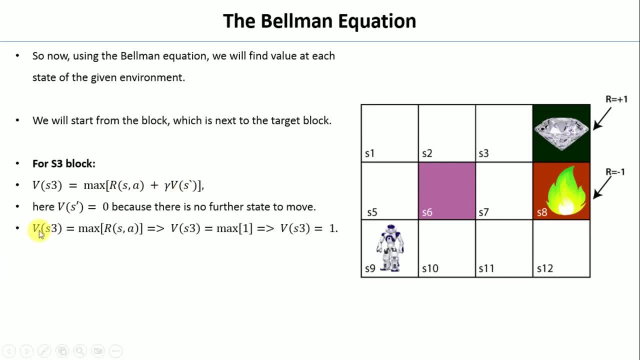 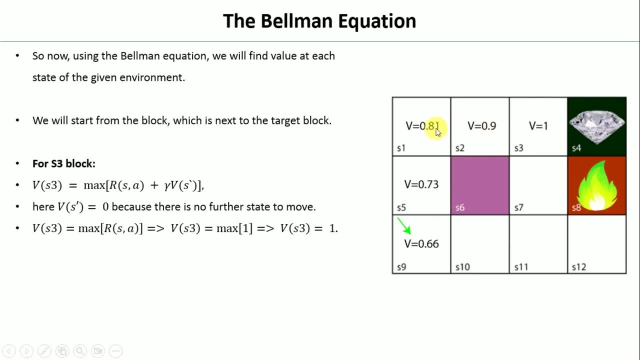 we have performed here. So if you put all those particular values, phi S3 will become the 1 in this particular case. so i will put that particular one over here. similarly, i have written the values for other states also. we will try to calculate step by step. in this case, now we have done with s3. 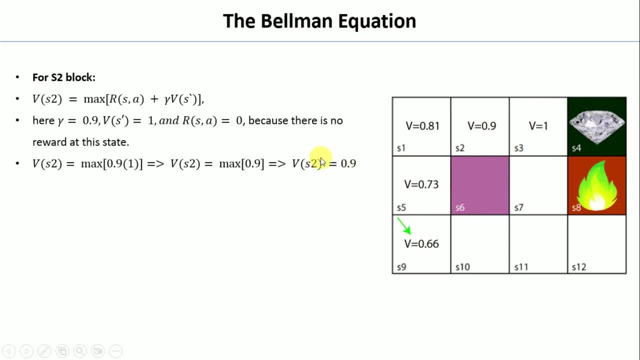 we will try to calculate the value for s2 the same equation we will use, that is, v? s2 is equal to maximum of rsa plus gamma or v s dash. so in this case rsa will become zero, because whenever you perform a right action, you don't get one here, because if you go through this particular goal, 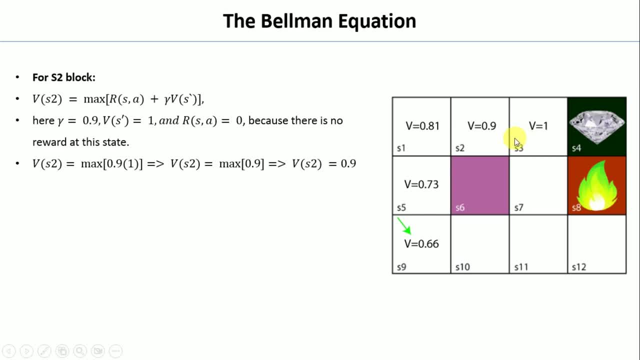 you will get one, but right now you are going to s3 here. so that's the reason: rsa will be zero. as i said earlier, gamma is equal to 0.9 v s dash. that's a previous state's value. what is the value we have here? one in this case. so it will become- this particular term will become zero. this will 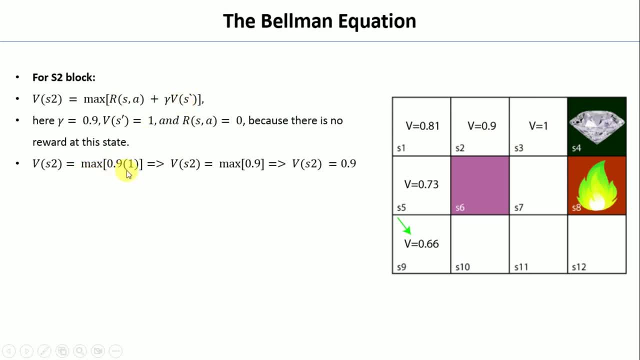 be 0.9 into one here. so that's the reason maximum of 0.9 into one v, s2 is equal and to 0.9 in this case. so that is what we got over here. similarly, we try to calculate it for s1 that. 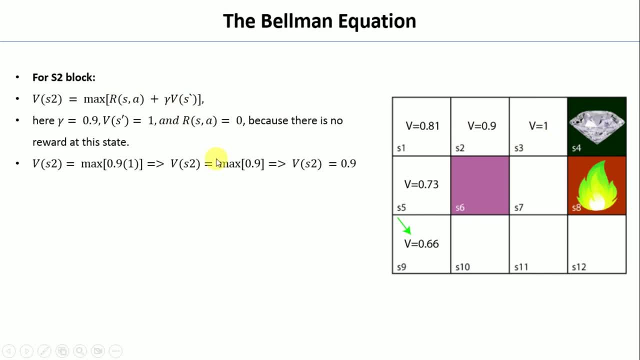 state's value. what is the value we have here? one in this case. so it will become this particular term will become zero. this will be 0.9 into 1 here. so that's the reason: maximum of 0.9 into 1 phi s2 is equivalent to 0.9 in this case. so that is what we got over. 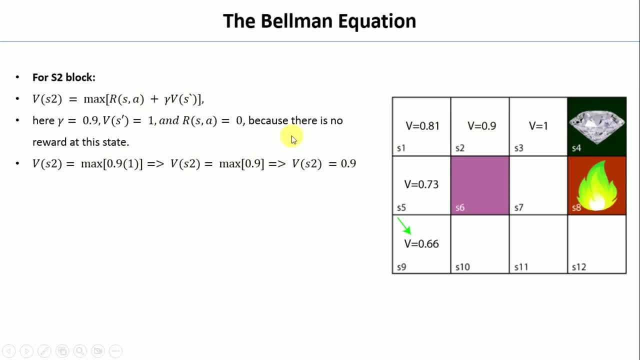 here. similarly, we try to calculate it for s1, that is, phi s1 is equivalent to maximum of rsa plus gamma phi s dash. again, rsa is equivalent to zero. here also, gamma is 0.9, which is known to us. the previous state value is equal to 0.9. phi s1 is equivalent to 0.9. phi s2 is equivalent to 0.9. 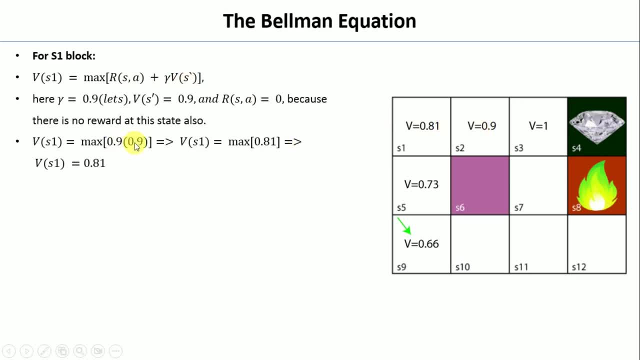 so if you put that particular thing 0.9 into 0.9, it will become 0.81. phi s1 is equivalent to 0.81 here, so that's the value i have written here. similarly we will calculate it for s5. here also the rsa is: 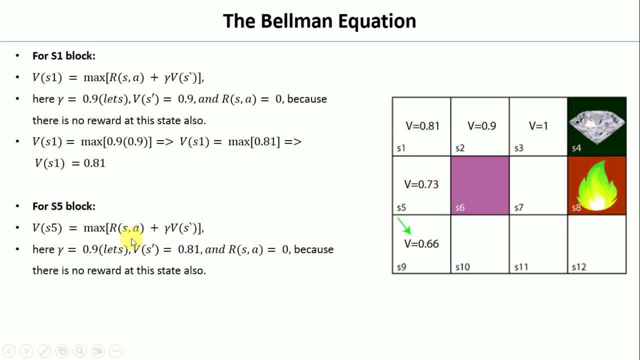 zero, but the previous value is equivalent to 0.81. 0.81 multiplied by 0.8 is equal. 0.9 is equivalent to 0.73 in this case. so that is, s5 is equal to 0.73. here now i will go to s9. here now the same. 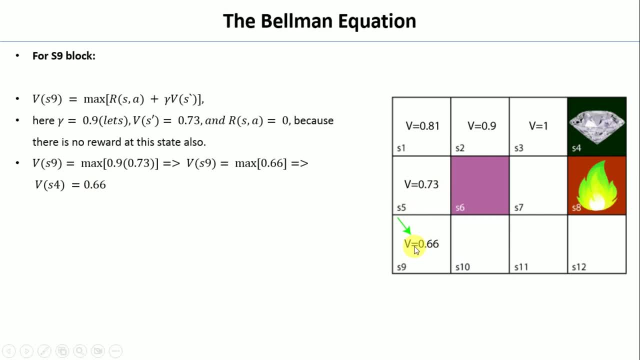 approach we will follow and we will get 0.66 for s9 in this case. now we will try to calculate it for s10, s10- we will get it 0.59. so that is what i have written here. similarly, we will go to s11. 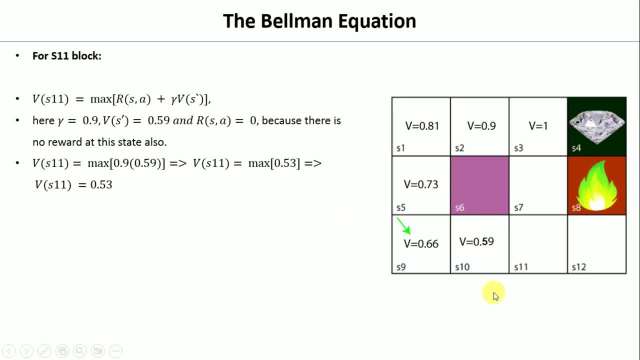 in this case. so if i go to s11, i will get 0.53 over here- the same approach i have followed, and then i will go to s12, i will get 0.48 over here. so i have started. in this case, i have gone. 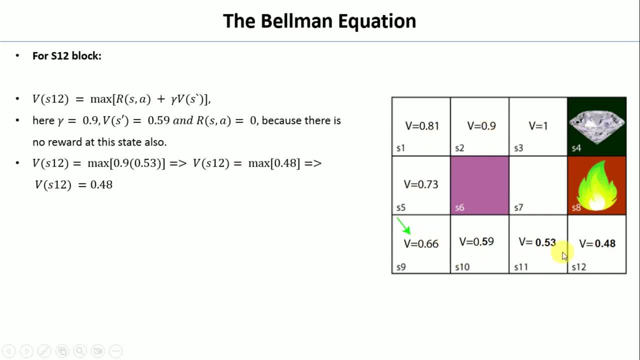 through this particular path. i have got all the values here. now we have one more cell here that is s7, so i cannot go left side. i cannot go right side, because this is the fire here. if i go down, i am getting. the previous state value is equal to 0.53. 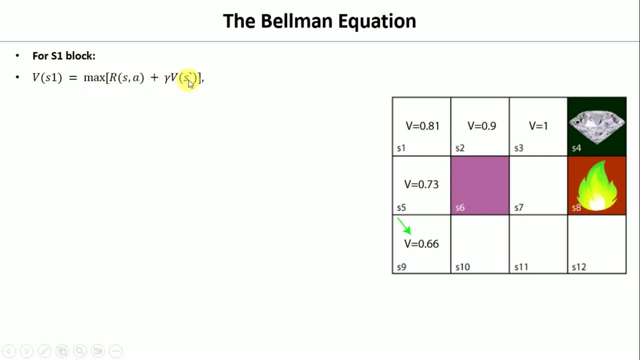 is phi s1 is equal to maximum of rsa plus gamma v s dash. again, rsa is equal to zero. here also, gamma is 0.9, which is known to us. the previous state value is equal to 0.9, so if you put that particular thing 0.9 into 0.9, it will become 0.81. phi s1 is equal to 0.81 here. so that's the value. 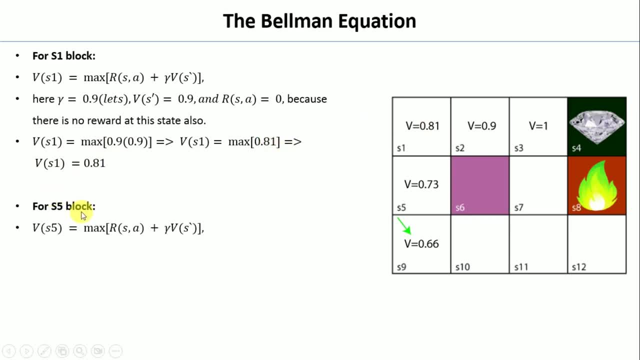 i have written here. similarly, we will try to calculate the value of rsa, which is equal to 0.9. similarly we will calculate it for s5. here also, the rsa is 0, but the previous value is equal to 0.81. 0.81 multiplied by 0.8 is equal. 0.9 is equal to 0.73 in this case. so that is. 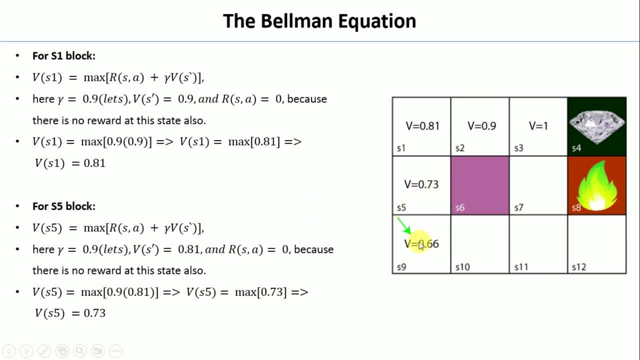 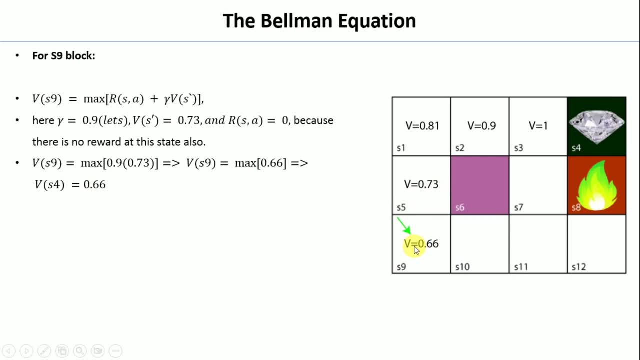 s5 is equal to 0.73 here now i will go to s9 here now. the same approach we will follow and we will get 0.66 for s9 in this case. now we will try to calculate it for s10. we will get it 0.59. so that is what i have written here. similarly, we will go to s11 in this. 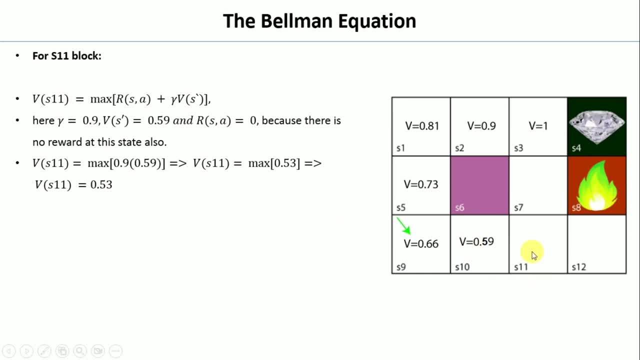 case. so if i go to s11, i will get 0.53 over here- the same approach i have followed- and then i will go to s12, i will get 0.48 over here. so i have started in this case, i have gone through this. 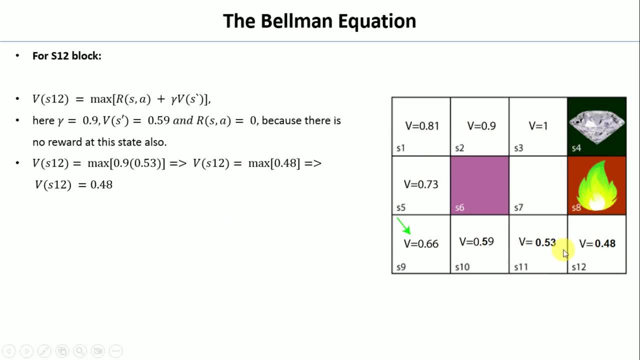 particular path. i have got all the values here. now we have one more cell here that is s7, so i will go to s12, because this is the fire here. if i go down i am getting. the previous state value is equivalent to 0.53, but if i consider the previous state is equivalent to s3. this is one here so that 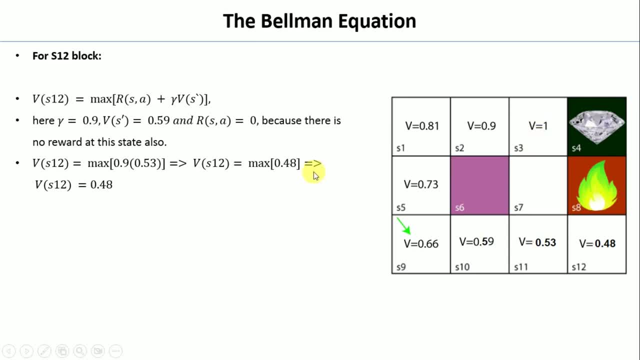 is a maximum, so i have to consider this one here. so for s7 you can say that the previous state is equivalent to 1, and then rsa is of course 0 here, because we cannot go from s7 to s4 over here. so 0.9 into 1 we can. 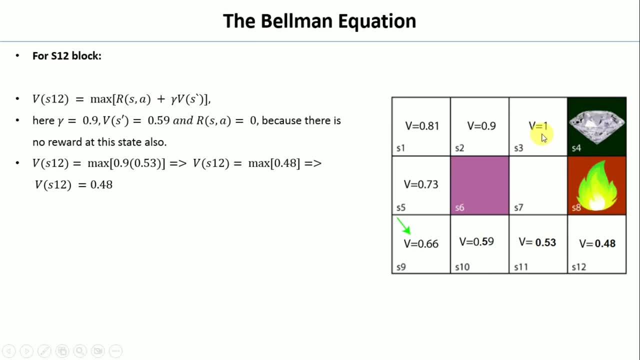 but if i consider, the previous state is equal to s3. this is 1 here. so that is a maximum. so i have to consider this one here. so for s7 you can say that the previous state is equal to 1, and then rsa is of course 0 here, because we cannot go from s7 to s4 over here. so 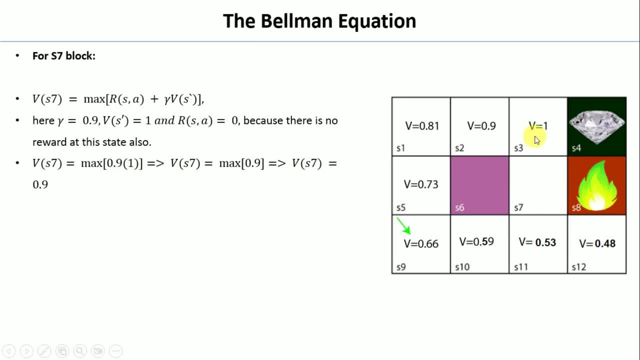 0.9 into 1. we can consider here: the previous state value is equal to 1 multiplied by 0.9. that is the gamma value. we will get 0.9 over here. now there is one more thing we need to consider while calculating s11. we have considered this path. 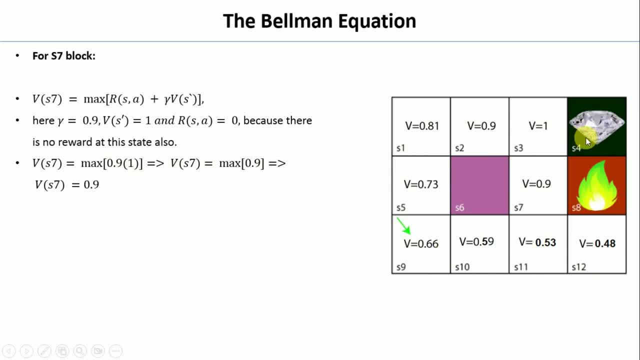 this is not the only path, what we have here. if you want to reach this particular s4 from s11, you can follow this path also. so we will try to calculate s11 by considering this one as the previous state rather than considering this one as the previous state in the earlier case we have. 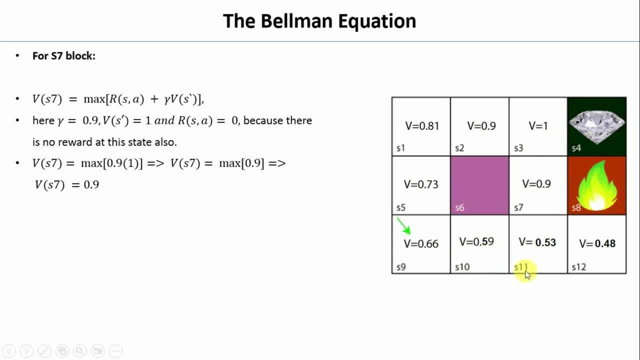 considered s10 as the previous state for s11. now we will try to consider s7 as the previous state and then we will see whether there is a modification to this particular value or not. so we will try to get maximum value over here. so i will try to calculate s11 one more time. 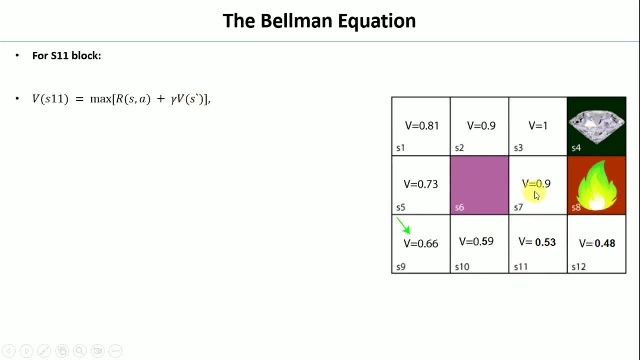 rsa is 0, of course, phi s dash, i will consider this one now. that is 0.9. multiplied by gamma, that is 0.9, it will become 0.81 in this case. so this particular 0.81 is greater than 0.53. so we will. 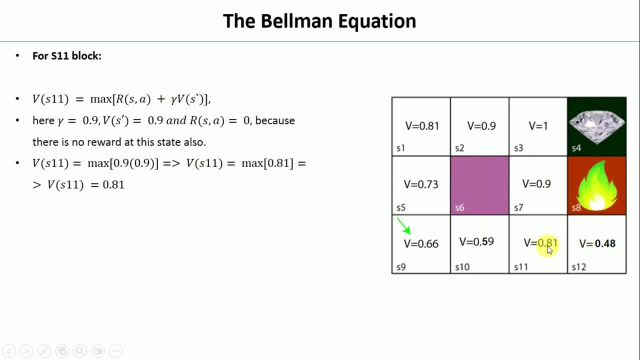 consider that as the value over here. now, when you consider 0.81 as the value over here, we have to consider s12 also, because while calculating s12 we have considered this as the previous state. now we will see and then calculate it one more time. so we s10 as well as s12- both we have to. 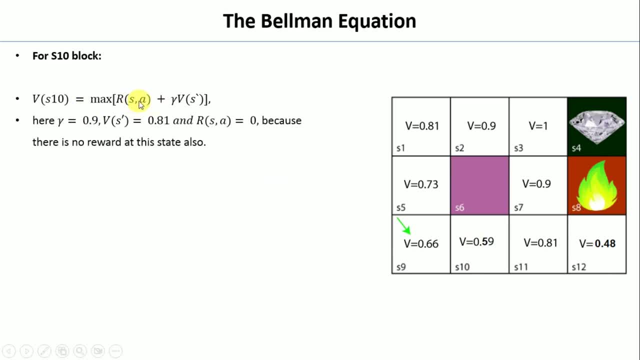 calculate s10. if we can calculate here again, rsa is equal to 0, that's for sure. this one is 0.81 multiplied by gamma. that is 0.9. that will become 0.73. previously i have written this 0.59, now it. 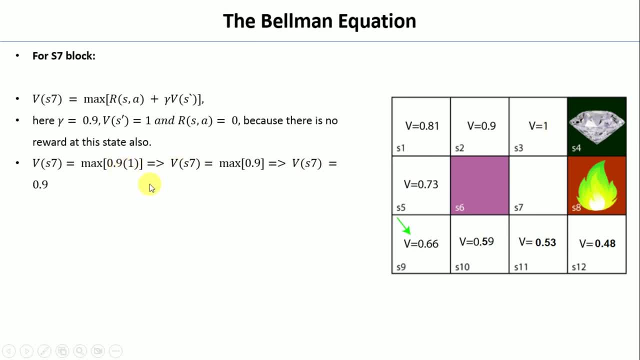 consider here: the previous state value is equivalent to 1 multiplied by 0.9. that is the value we will get 0.9 over here. now there is one more thing we need to consider while calculating s11. we have considered this path. this is not the only path, what we have here, if you want to reach. 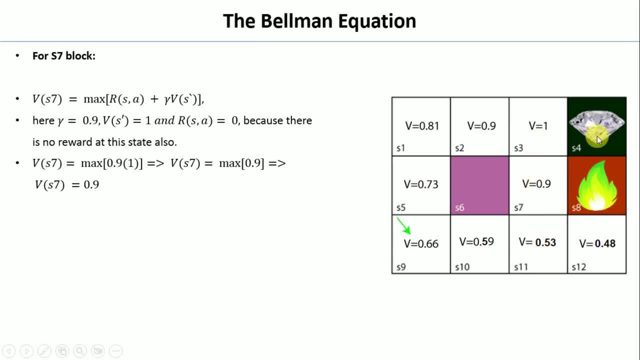 this particular s4 from s11. you can follow this path also, so we will try to calculate s11 by considering this one as the previous state rather than considering this one as the previous state. in the earlier case, we have considered s10 as the previous state for s11. now we will try to consider s7 as the previous state. 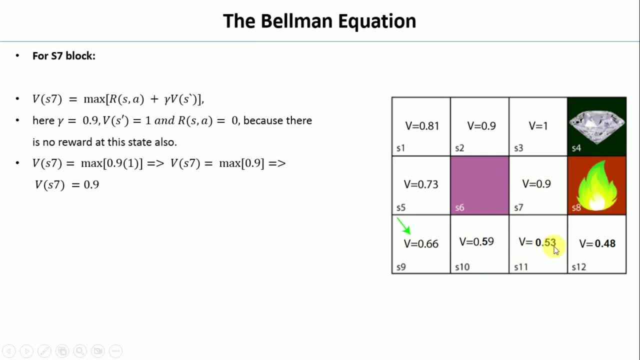 and then we will see whether there is a modification to this particular value or not. so we will try to get maximum value over here. so i will try to calculate s11 one more time. rsa is 0, of course. phi s dash, i will consider this one. now, that is 0.9 multiplied by gamma, that is 0.9. it will become: 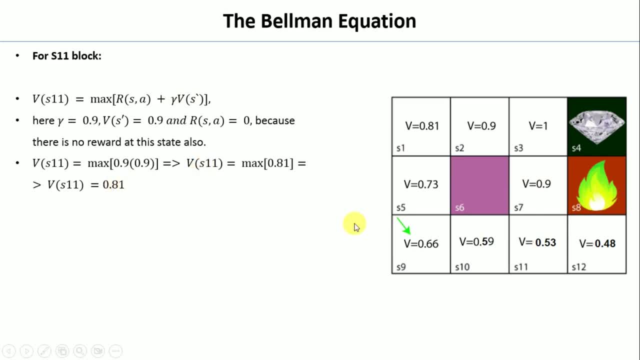 0.81 in this case. so this particular 0.81 is greater than 0.53, so we will consider that as the value over here. now, when you consider 0.81 as the value over here, we have to calculate the s12 also, because while calculating s12, we have considered this as the 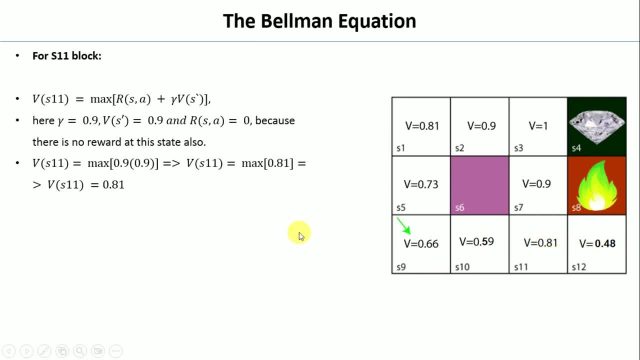 previous state. now we will see and then calculate it one more time. so we s10 as well as s12, both we have to calculate. s10, if we can calculate here again, rsa is equal to 0, that's for sure. this one is 0.81. multiplied by gamma, that is 0.9, that will become 0.73. 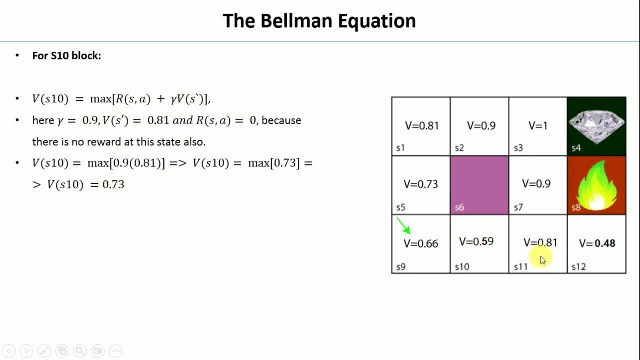 so this is the best option over here. so i will replace this with 0.73 in this case. the same thing. we have to follow this direction also, unless and until we will get the the least value. or you can say that if you are getting a better value, replace it over here. 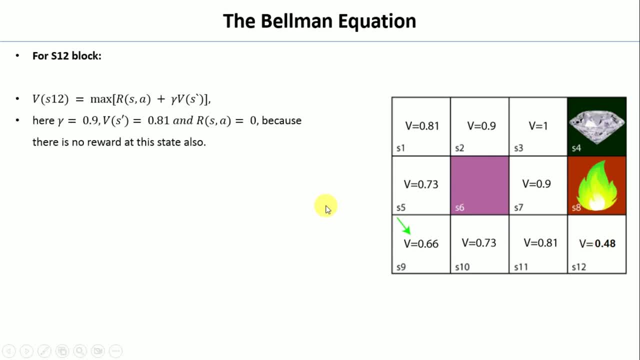 now we will try to calculate it for s12 also. if i do the calculation for s12, i am getting 0.73 if i consider this one as the previous state. so if i consider this 0.73, that is better than this particular 0.78 for 48. so definitely it will be the best. 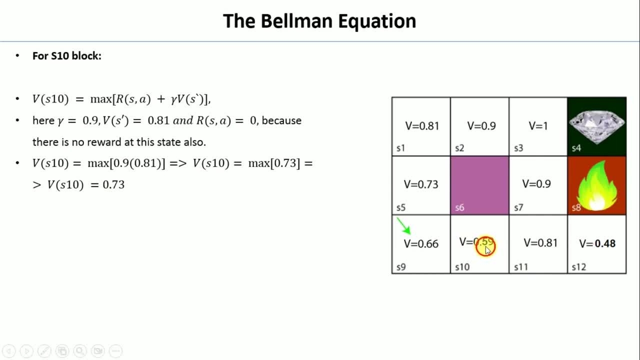 is 0.73, so this is the best option over here, so i will replace this with 0.73 in this case. the same thing. we have to follow this direction also, unless and until we will get the the least value. or you can say that if you are getting a better value, replace it over. 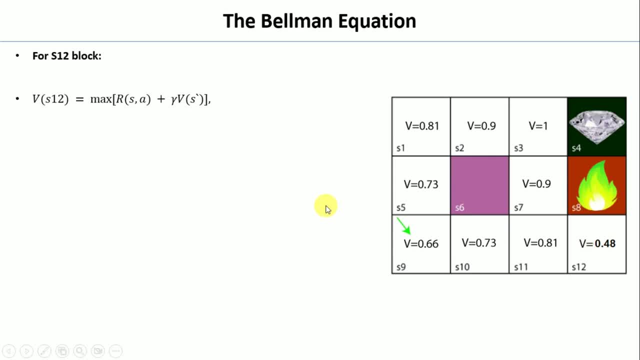 here now we will try to calculate it for s12 also. if i do the calculation for s12, i am getting 0.73, if i consider this one as the previous state. so if i consider this 0.73, that is better than this particular 0.78 for 48. so definitely it will be 0.73. and if i do the calculation for s12, i am. 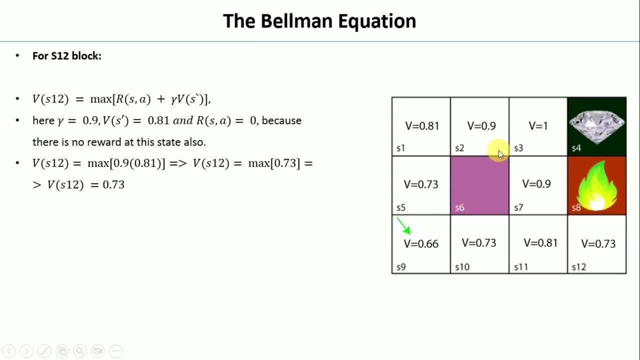 getting the best value over here. the same thing. we have to repeat it again and again, unless and until the we will get the final values for each and every state over here. now, once you get these particular values, let us say that the robot is present in any state it can reach this particular. 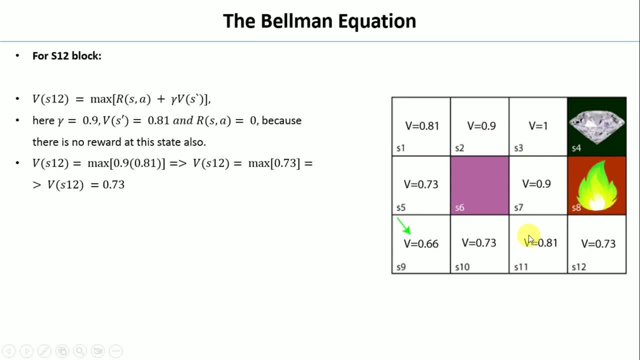 goal state by considering the optimal path over here. let us assume that the agent is present in s1. if it is present in s1, it will try to check the value of the neighboring cells. so if it consider the right moment, it will get 0.9 as the value. if it considers the down movement, it will get 0.73. 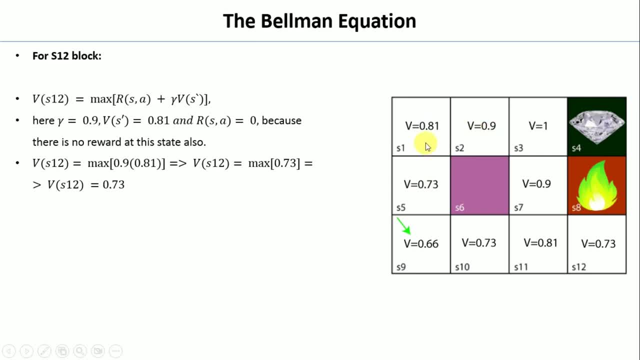 so this is the better option over here. so it will go to this particular side, that is, s1 to s2. so when it goes to s2 it will try to find the again the possible paths. so it it has two possibilities: one is right and one more is you can say that the left here. 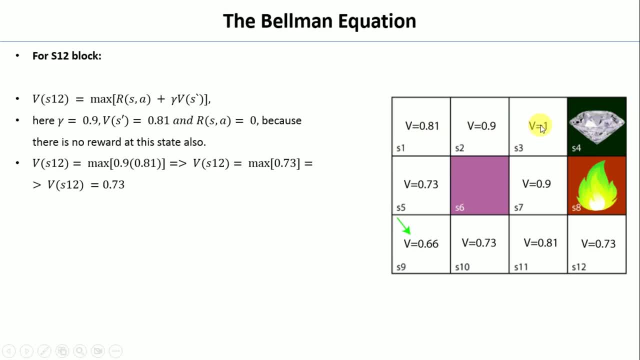 so left is 0.81, right is one, so one is the better option. so it will go through this particular s3 here. so s1 to s2, s2 to s3 and then s3 to gold state it is. one can reach directly over here when it is present in this s10. you can see when it is present in s10. 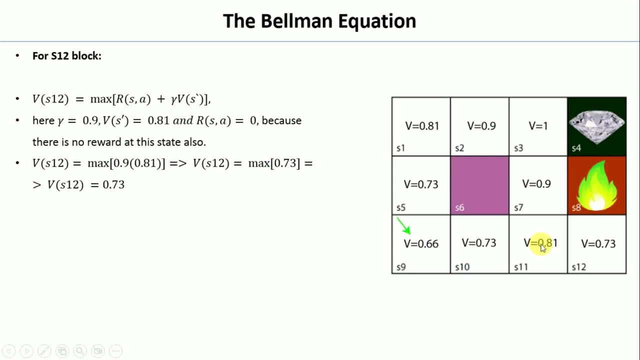 it has two possibilities: it can go left or it can go right here. okay, so when it is present in s10, it cannot go left because the value is 0.66, as the value on the right side is more in this case. so 0.81 is better than 0.66, so it will go right side here. so when it goes to s11, again there are 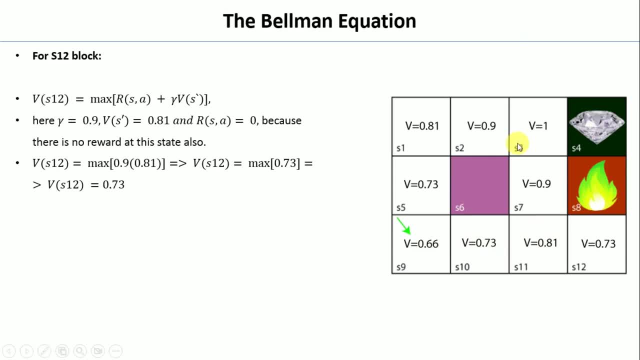 three possibilities: left, right, and what we can say, that the up here left is 0.73, right is 0.73, up is 0.9. so 0.9 is better option here. so it will go up in this case when it is present in here. 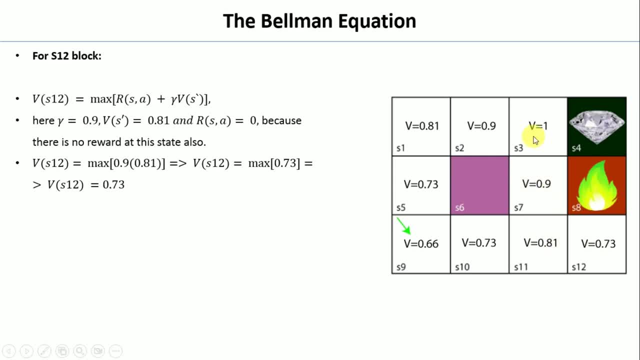 it cannot go left or right, it can go down or it can go up here. so upper value is one that is better than the lower one. so it will go to this s3 and from s3 it can easily go through this particular s4 over here. so whenever agent is present in any 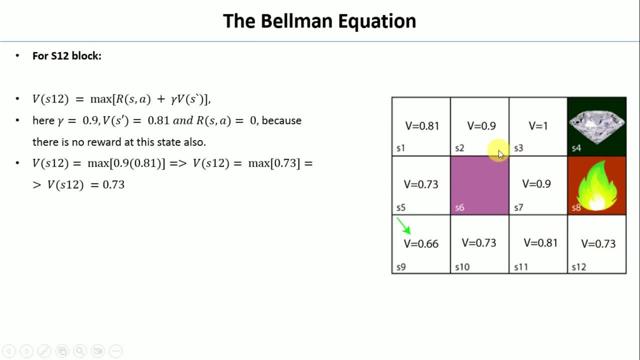 value over here the same thing. we have to repeat it again and again, unless and until the we will get the final values for each and every state over here. now, once you get these particular values, let us say that the robot is present in any state it can reach this particular goal state. 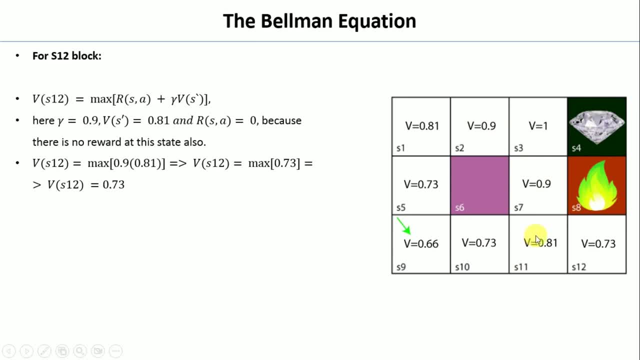 by considering the optimal path over here. let us assume that the agent is present in s1. if it is present in s1, it will try to check the value of the neighboring cells. so if it consider the right moment, it will get 0.9 as the value. if it considers the down moment, it will get 0.73. 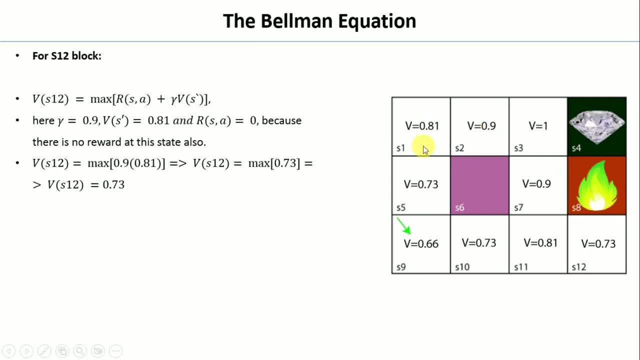 so this is the better option over here. so it will go to this particular side, that is, s1 to s2. so when it goes to s2 it will try to find the again the possible paths. so it it has two possibilities: one is right and one more is you can say that the left here. so left is 0.81, right is 1. 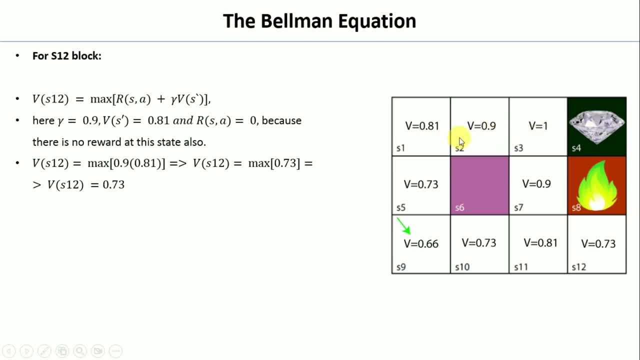 so it will go to this particular option. so it will go through this particular s3 here. so s1 to s2, s2 to s3 and then s3 to goal state. it can reach directly over here. when it is present in this s10, you can. 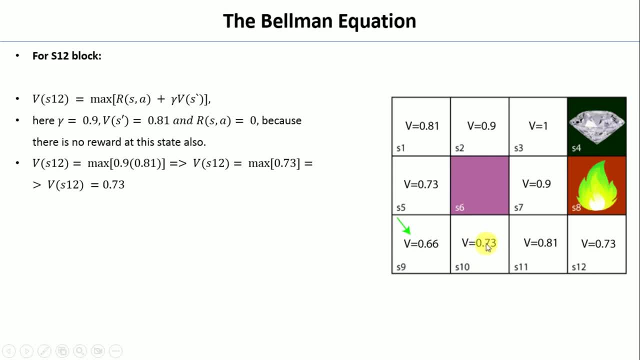 see, when it is present in s10, it has two possibilities: it can go left or it can go right here. okay, so when it is present in s10, it cannot go left because the value is 0.66, as the value on the right side is more in this case. so 0.81 is better than 0.66, so it will go right side here. so 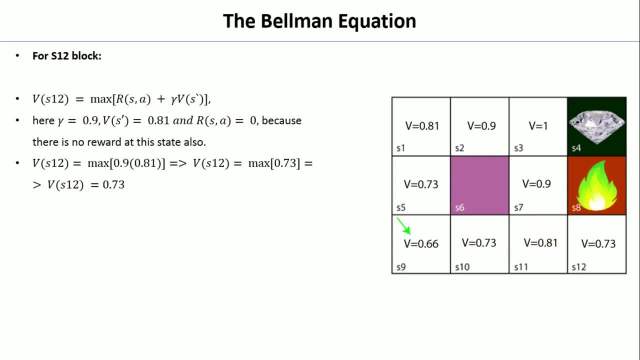 when it goes to s11. again, there are three possibilities: left, right and what we can say: that the up here left is 0.73, right is 0.73, up is 0.9. so 0.9 is better option here, so it will go up. 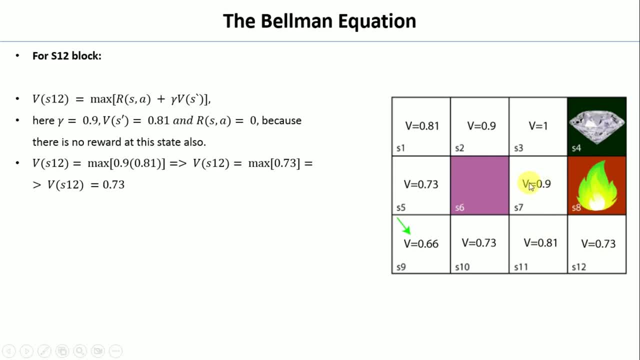 in this case, when it is present in here, it cannot go left or right, it can go down or it can go up here. so upper value is one that is better than the lower one. so it will go to this s3 and from s3 it can easily go through this particular s4 over here. 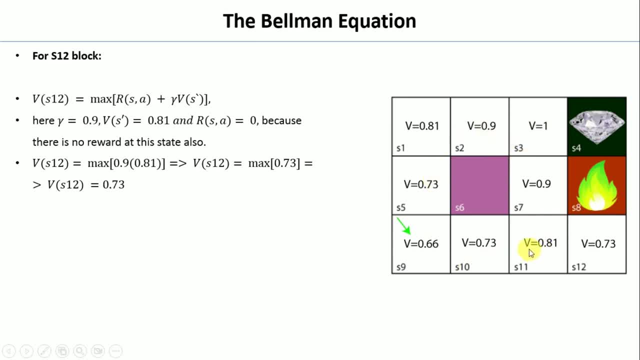 agent is present in any cell over here, it can find an optimal path and it will reach this particular goal state perfectly without any problem in this case. so this is how we can use bellman equation to assign values to each and every cell using this particular cell agent can go. 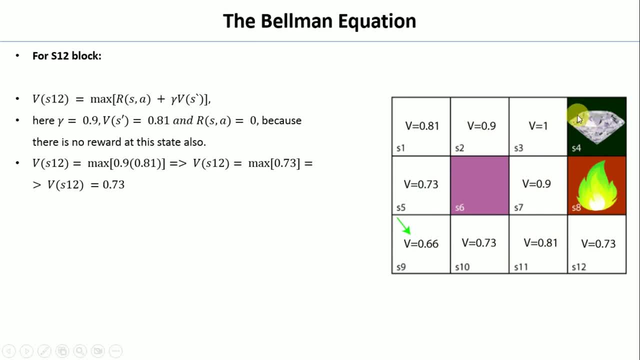 particular s4. it is present in this particular s4 with option 3, so it can go up in this case, alright, and here is another option. then we connect the genGILEays, which the other options can go cell over. here it can find an optimal path and it will reach this particular goal state. 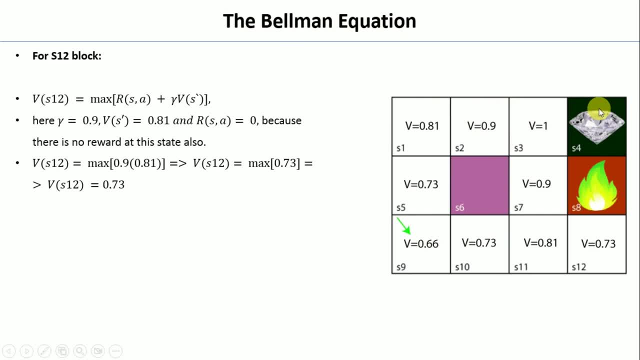 from any state to goal state with an optimal path over here. so in this video i have discussed how we can use bellman equation in reinforcement learning. i hope the concept is clear. if you like the video, share with your friends. press the subscribe button for more videos.